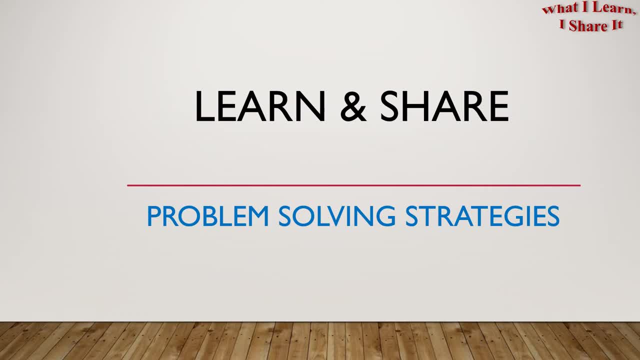 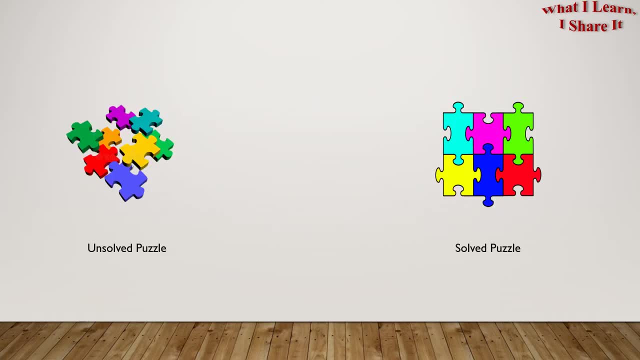 Hello friends, Welcome to Learn and Share. In this video, we'll be discussing the problem-solving strategies. So let's get started. How do we solve a puzzle? We make a plan and we use the strategy to put the pieces together and complete the puzzle. 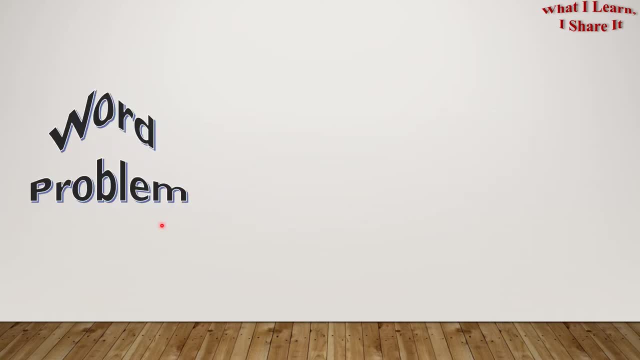 In the same way, we have a word problem here which looks very, very, very scary to us. We have to use this strategy to move towards a very good-looking solution. Let's look at the various problem-solving strategies. The first one is draw pictures or blocks. 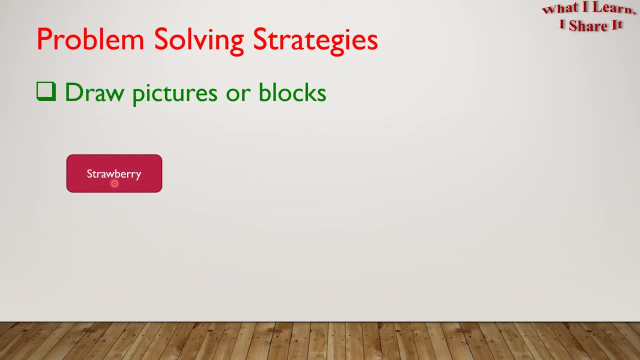 We can represent some amount of strawberries by one block and double the amount of blueberries by two blocks. You can see the examples in our playlist for third grade. Make an organized list. We can use an organized list to find all the combinations of one primary color and one secondary color. 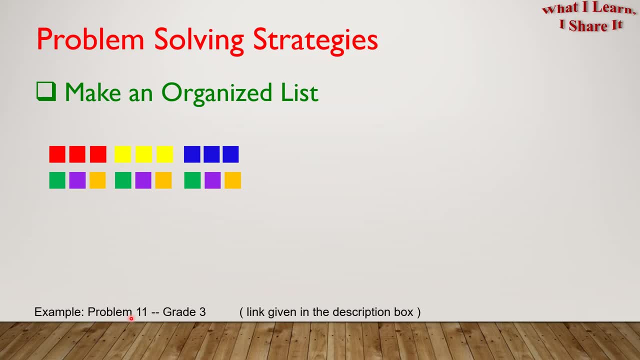 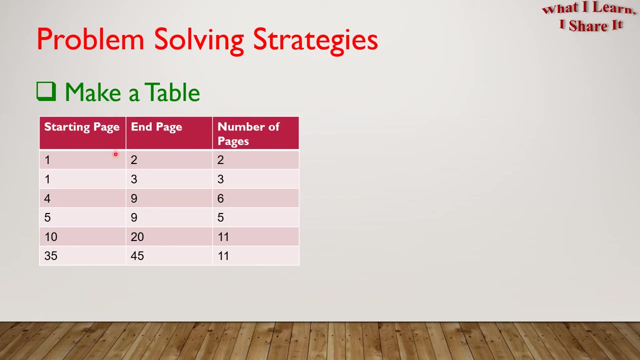 This is the strategy we used in problem 11 from grade 3.. Our next strategy is make a table. We use this strategy to find the total number of pages when the starting page and end page are given. Remember problem 10 from grade 2?? 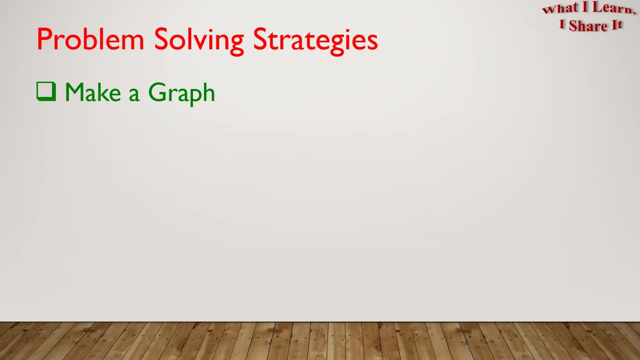 We use this strategy there. We use this strategy to find the reading time and math time in the months of January, February, March and April. This is an example from problem 13, grade 3.. So our next strategy is act it out or use objects. 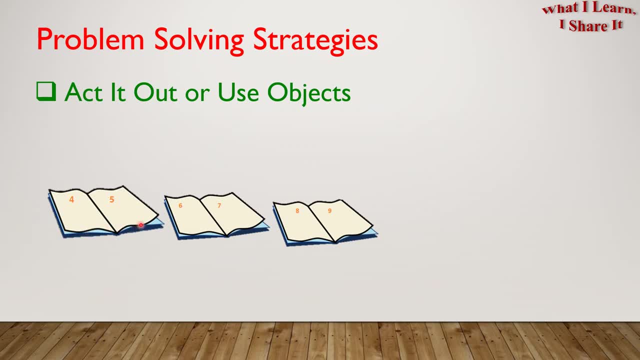 I use this strategy to understand the problem of page numbers. You can also refer to problem 10 for grade 2.. Link is given in the description box. Looking for a pattern, As we see here that every week the number of coins is increasing by one.